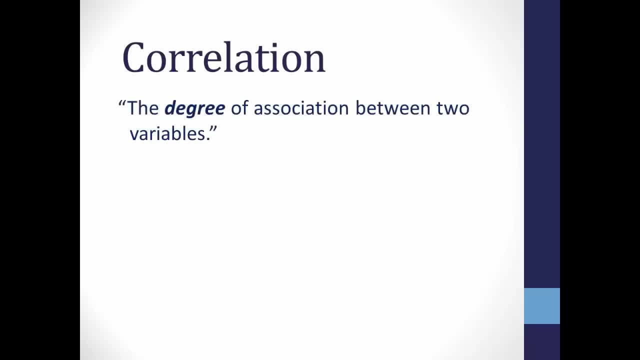 Correlation has been defined as the degree of association between two variables or a measure of the strength of association among and between variables. Correlation is not defined as causation. At the risk of repeating myself, correlation is also known as association, Say. for example, we find that males are more likely than females to classify themselves. 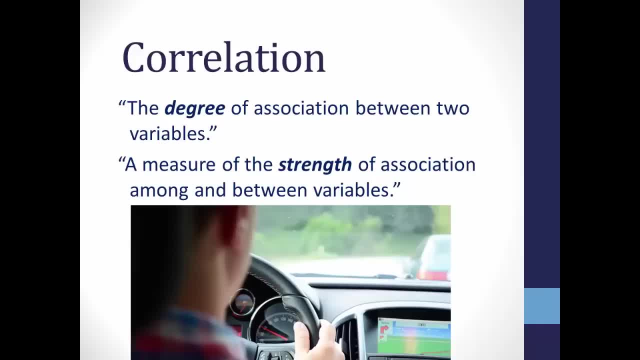 as better than average drivers. That doesn't mean that being born male causes you to be a better driver. Sorry guys, But it does mean that there is an association, a correlation or a relationship between a person's sex and their perception of driving prowess Another. 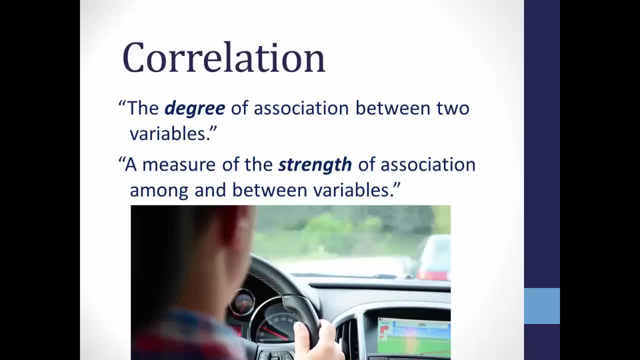 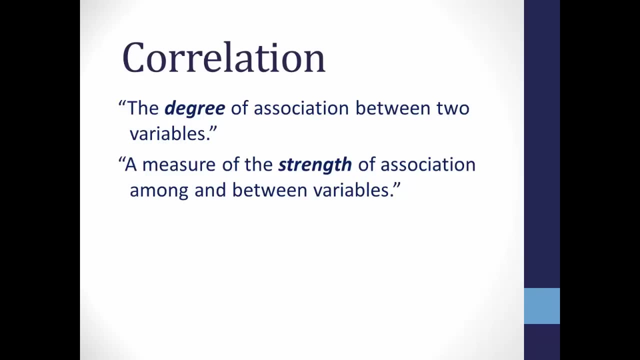 example might be that as number of years of driving experience increases, the number of accidents, tickets etc. decreases. Driving experience, then, could be correlated or associated with safer driving, Or at least that's what auto insurance companies are banking on. This video will focus on correlation and, to a lesser degree, regression, In particular. 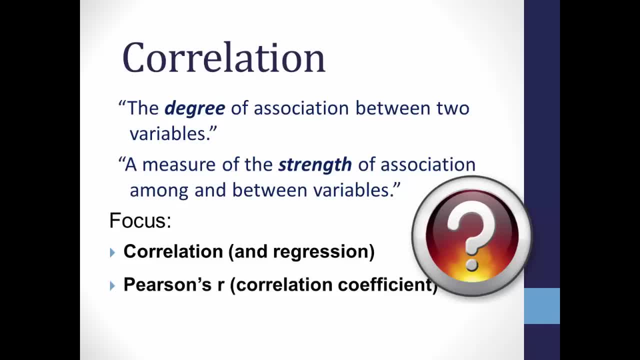 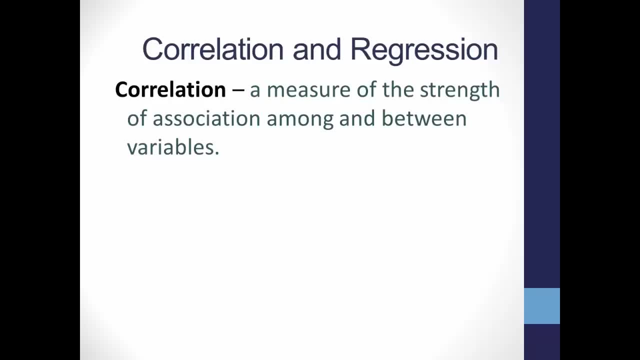 we will examine Pearson's r correlation coefficient, with a mention of Pearson's r squared, which is the coefficient of determination. As we said earlier, correlation is a measure of the strength of association among and between variables. You first attempt to answer the question: is there any relationship between two or more variables? You can do this with: 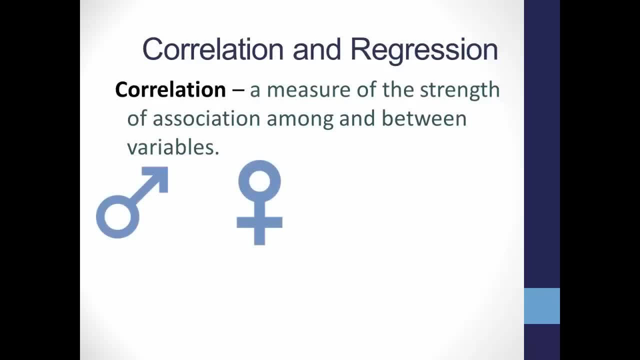 nominal level variables, or you can do this with a number of variables, or you can do this with a number of variables, such as: is a person's sex related to or associated with or correlated with, pregnancy? Now, being female, for example, would not cause. 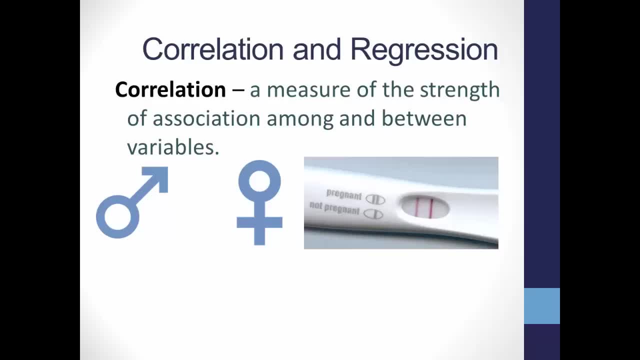 you to become pregnant. The two variables are, however, strongly correlated. There is a relationship between them. However, you'll usually find correlation analysis when you are measuring two continuous level variables, such as amount of time running on a treadmill, measured as a continuous variable, and calories burned or calories burned. You can then measure. 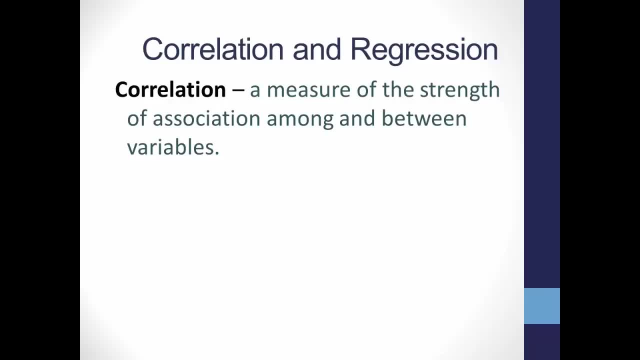 the number of calories burned, also measured as a continuous variable. We use a correlation coefficient with continuous level variables to express the strength of that association. Is the connection or relationship a strong one, a weak one, or is it non-existent? 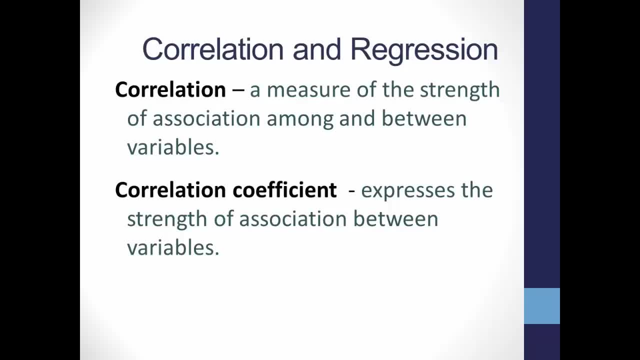 Just knowing that a relationship exists between variables may not be enough. If you want to predict the value for one variable based upon the value of another variable, you will need to use regression analysis. With correlation, we are just looking for an association or a connection between random variables, while with regression you are 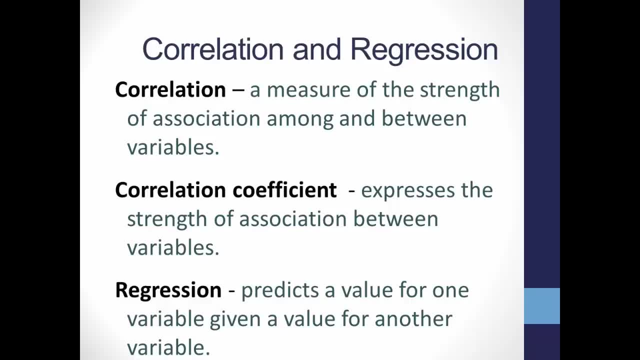 looking to see that if you change one variable, a fixed variable, you can predict a change in the other random variable. We use Pearson's r, also known as Pearson's Product Moment Correlation Coefficient, for correlation and r squared for regression. Don't worry. 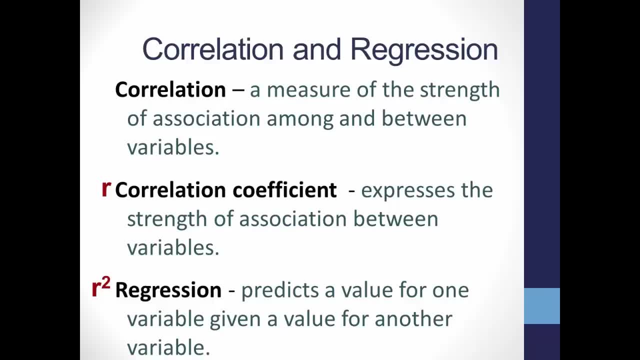 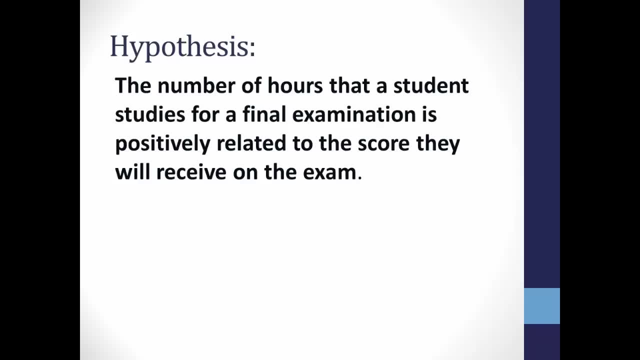 right now. if you don't 100% understand the difference between the two, Just know that they exist as we move on. I'm going to give you a couple of examples here. Assume that you have a hypothesis that says the number of hours a student studies for a final exam. 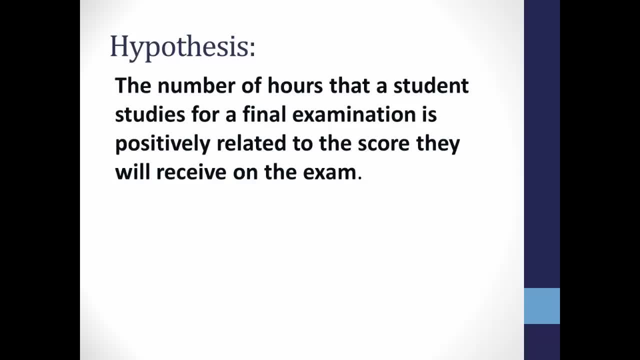 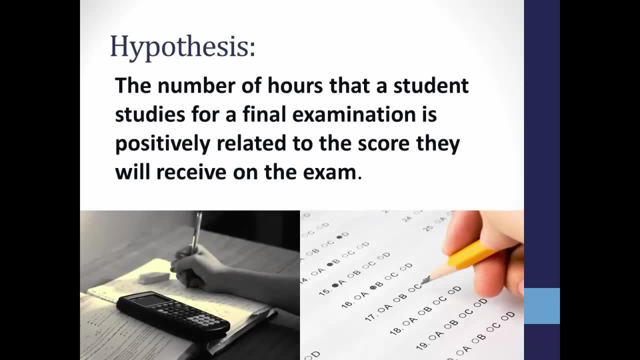 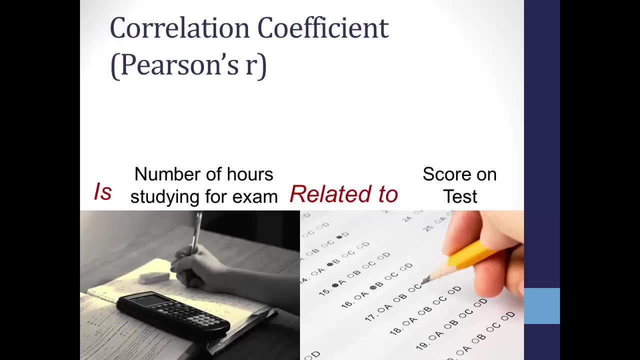 is positively related to the score they will receive on that exam. Two variables, both of which are continuous level variables- number of hours studying and score on the exam. You can calculate a mean on both of these variables To determine if a relationship exists between. 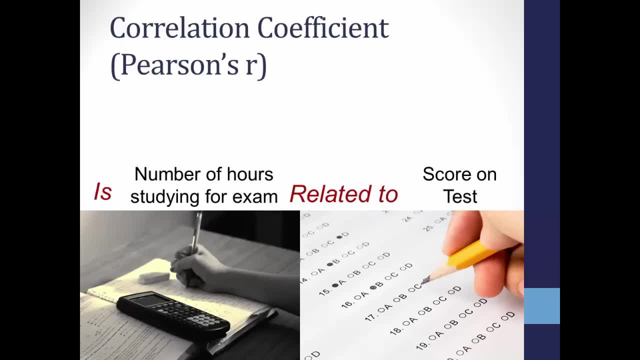 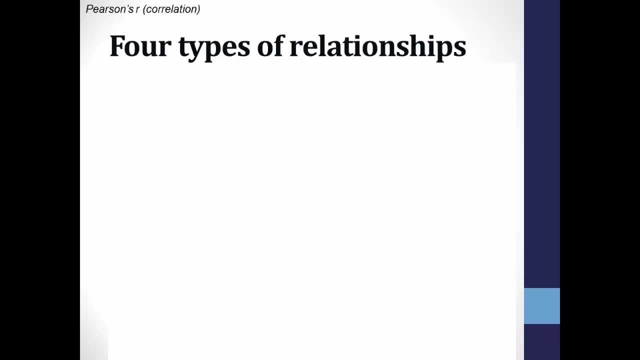 hours of study and exam score. you would calculate Pearson's R because it measures the linear relationship between two continuous level variables. They could be gathering interval or ratio level data. If you plotted out the data, there are four types of relationships that could exist. The first is the one you would probably expect for this example: a. 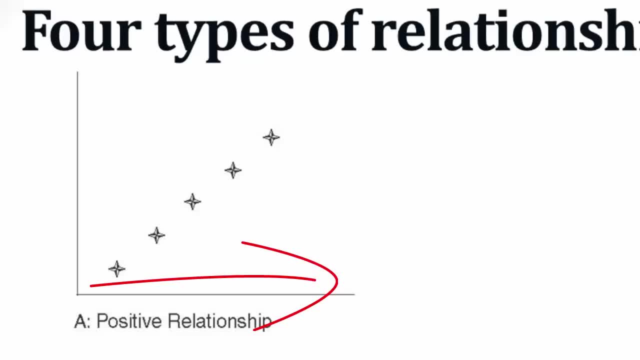 positive relationship: The more hours spent studying, the higher the score on the exam. There are a few perfect correlations, but many that are close, such as comparing the number of people who go to see a movie and resulting ticket sales- A negative relationship. 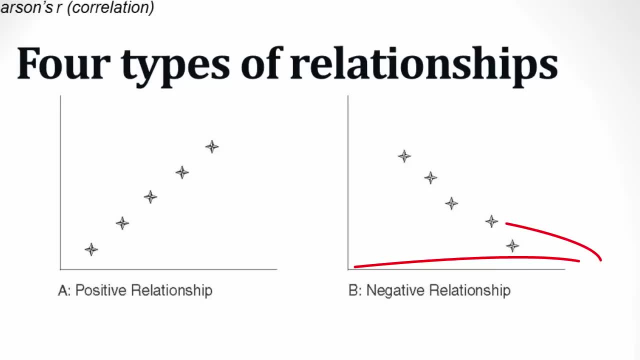 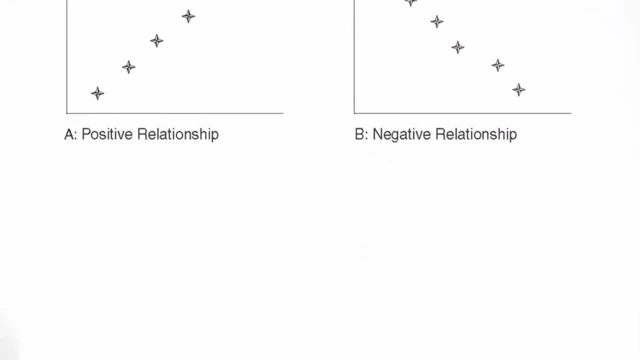 is the opposite: The more hours spent studying for an exam, the worse the score. Or, as a person's age increases, their agility level decreases. A curvilinear relationship might also exist. For this example, let's change the variables to anxiety level and preparedness. 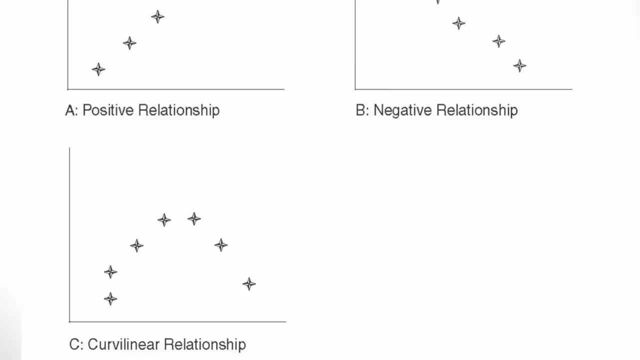 for a test. Those who are unprepared for a test may experience low anxiety levels when taking the test. They know they won't do well, so why sweat it? And those who are really prepared may experience low anxiety levels when taking the test. Those who are really 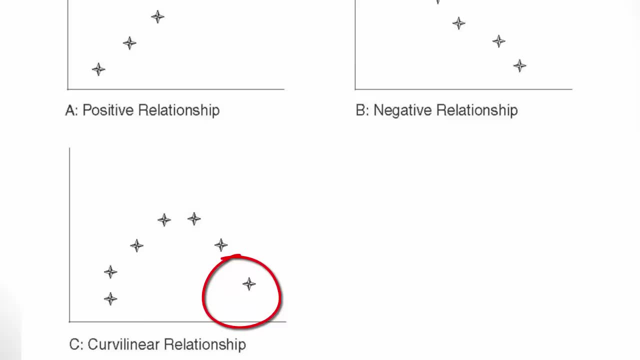 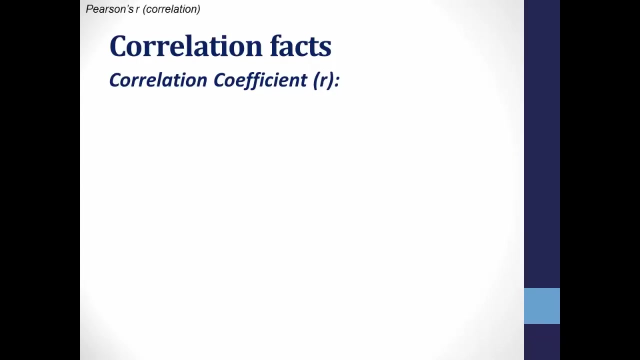 prepared may also experience low anxiety levels. They have it down cold, so why worry? But it's those in the middle who might experience higher levels of anxiety. And of course, there could be no relationship between the two variables. When you finish calculating Pearson's R, you'll end up with values ranging from negative. 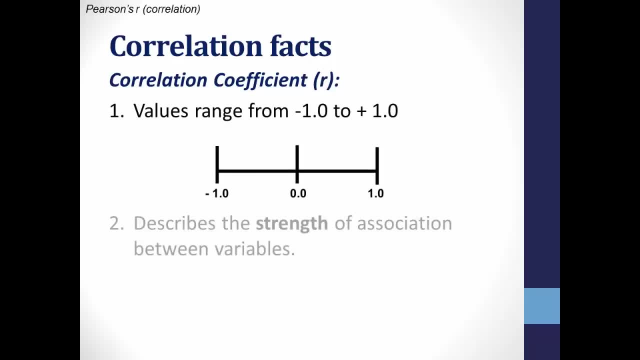 one to positive one. The value describes the strength of association between variables. The closer the Pearson's R statistic is to one, either negatively or positively, the stronger the relationship between the variables, And the positive and negative signs will tell you the direction of association between the variables. If it is a negative number, it's 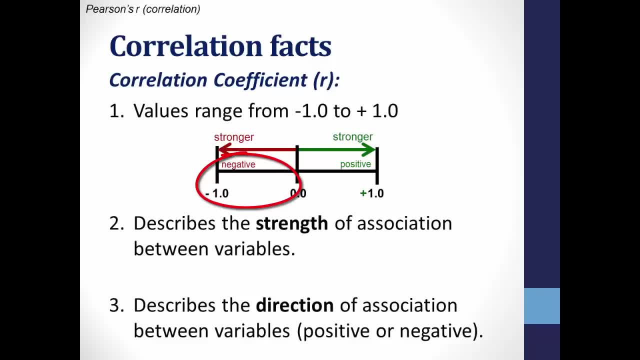 a negative relationship. For example, more hours studying could be negatively correlated with exam scores. The more you study, the worse you do. A positive number would mean that the more hours you study, the better you would do on the exam. But it's important. 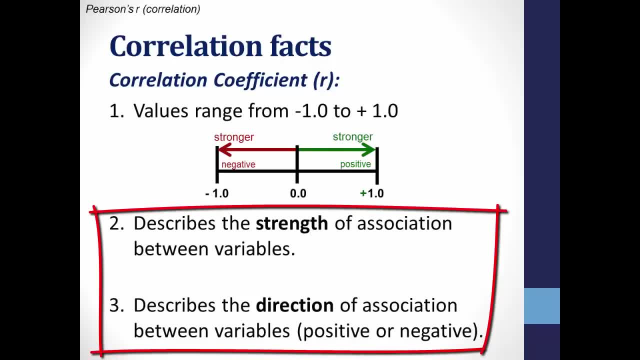 to pay attention to both number two and three here. A Pearson's R of 0.15 is the number of hours you study, and the number of hours you study is the number of hours you study. A Pearson's R of 0.15 is the number of hours you study. A Pearson's R of 0.15 is the number. 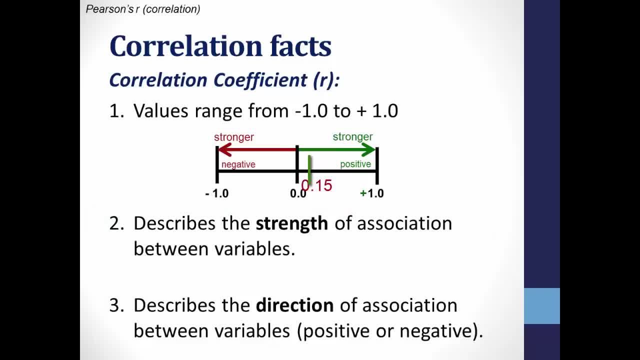 of hours you study, and the number of hours you study is the number of hours you study. If you were to use the information provided here, you'd have to be a bit more careful with the word correlation. The bottom line is that a Pearson's R of 0.15 would indicate: 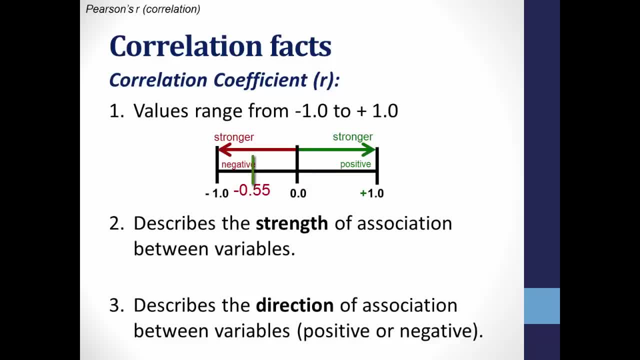 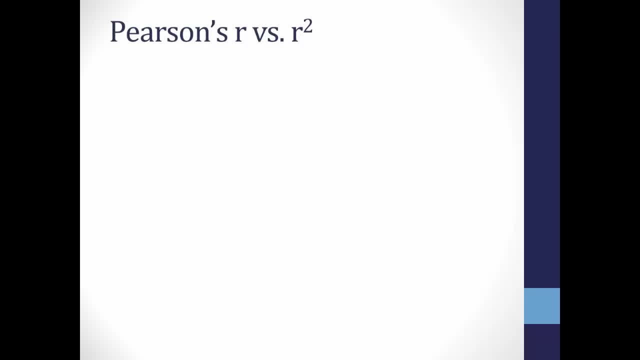 a weak positive correlation, while if you calculate a Pearson's R at negative 0.55, that means it's a stronger correlation, but in the negative direction You may hear Pearson's R and R squared. What's the difference? Pearson's R is correlation. 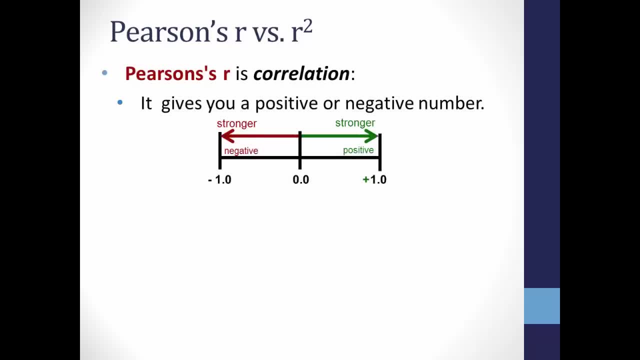 telling you the strength of association and whether it is a positive or negative correlation. R squared then is Very simply: taking the Pearson's R statistic and squaring it. It will always then be a positive number ranging from 0 to 1.0.. 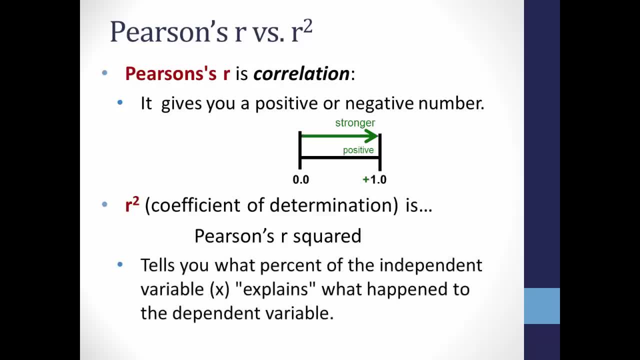 This tells you what percent of the independent variable, say hours of studying, explains what happens to the dependent variable, such as exam score. The closer R squared is to 1, the better the prediction. In other words, the better X explains what happens to Y. 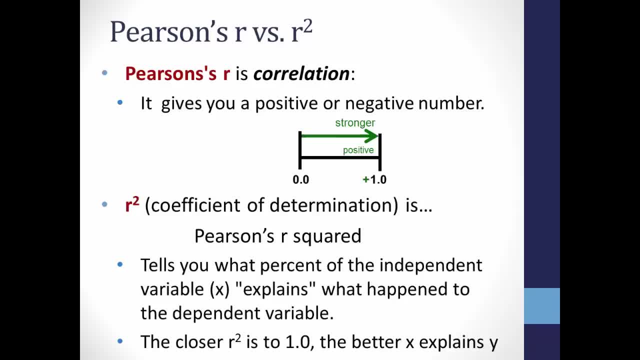 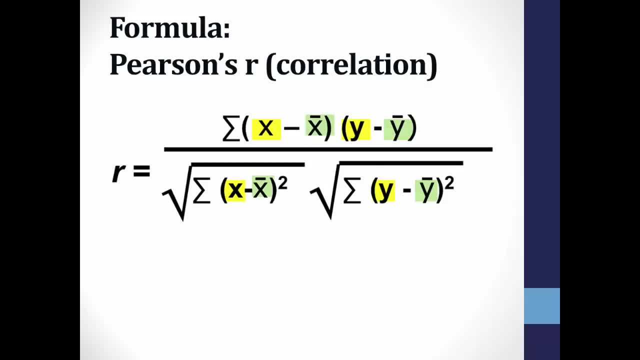 So R squared, then, is used for regression analysis. That takes us to the formula for Pearson's R. Notice that you really only need to know the scores for each group and the means for each group And degrees of freedom, which you need to look up the critical R value on a table to 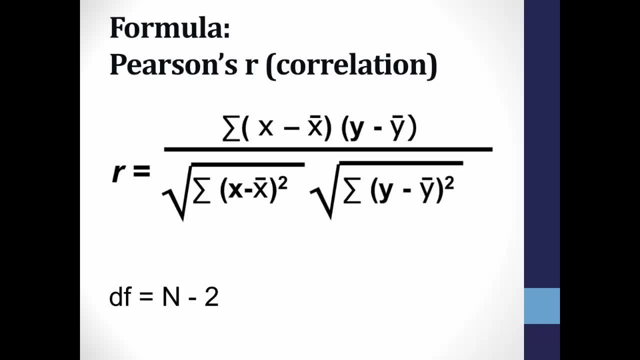 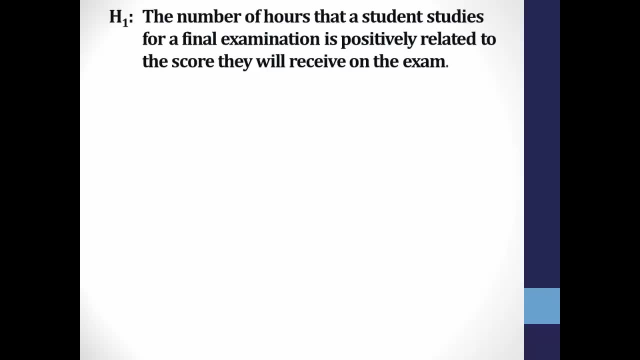 determine if your findings are indeed significant is the number of observations minus 2.. Back to our hypothesis that there is a correlation between the number of hours spent studying for an exam and the resulting score on the final examination, You gather data from seven students on the hours they studied, which we will call the X variable, and their 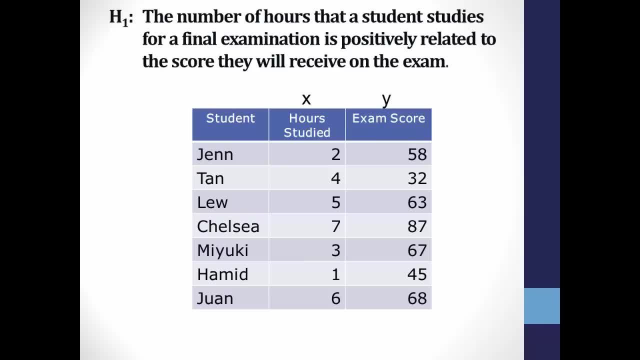 exam scores, or the Y variable. So the N for each variable is 7.. In total, however, you have 14 observations- 7 for the X variable and 7 for the Y variable, And you'll need to know this to calculate degrees of freedom. 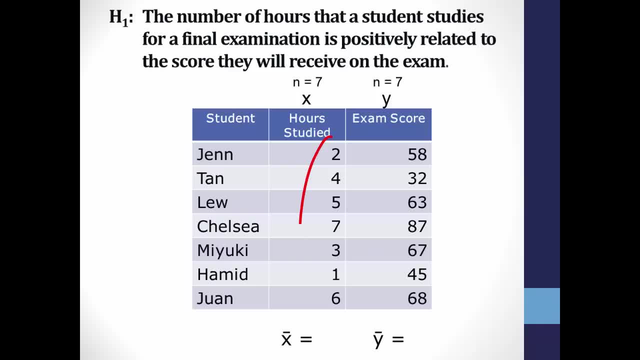 You can calculate the mean for each set of numbers. So, for hours studied, 2 plus 4 plus 5 plus 7 plus 3 plus 1 plus 6 equals 28, divided by 7, which is the N for the hours they studied. 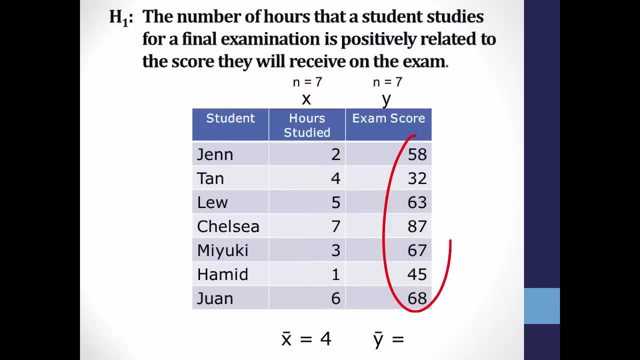 This is the answer for the X variable, which is 4.. Do the same thing for exam scores, the Y variable. You'll come up with 60 as the mean. So the mean of X is 4 and the mean of Y is 60.. 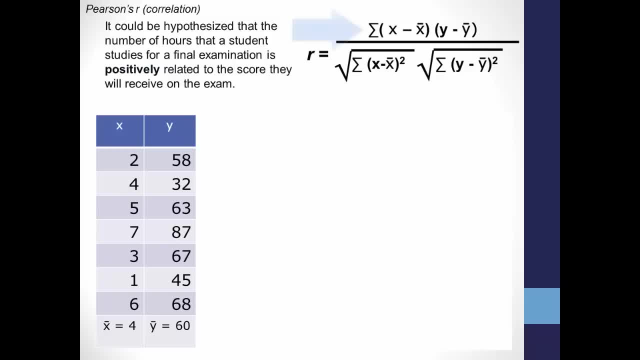 So now we have all we need to start doing our calculations. Look at the numerator of the formula. the sum of each score in the group minus the group mean You do this for the scores on the X variable number of hours and the Y variable score. 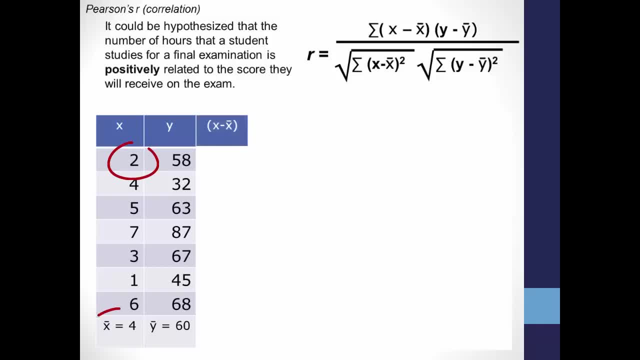 on the exam. So, starting with X, 2 minus the mean of X, which is 4.. 4 equals negative 2.. Then 4 minus the mean of x, 4, equals 0. Continue doing this for all the scores in the x group, And then do the same for y, 58 minus the mean of y, which 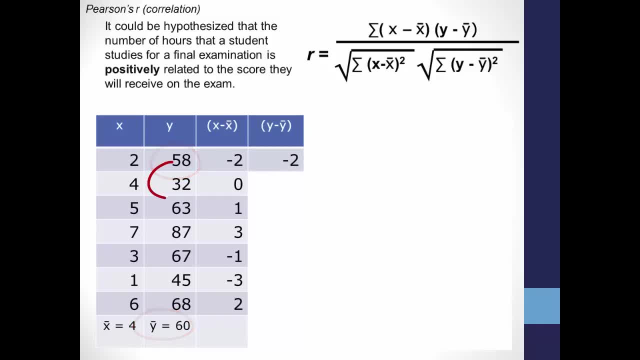 is 60, equals negative 2.. Then 32 minus the mean of y, 60, equals negative 28,, and so on. The formula tells us to multiply these two scores together, So you have negative 2 times negative 2, or 4.. Then 0 times negative 28 is 0,, and then so on. Sigma tells us to add: 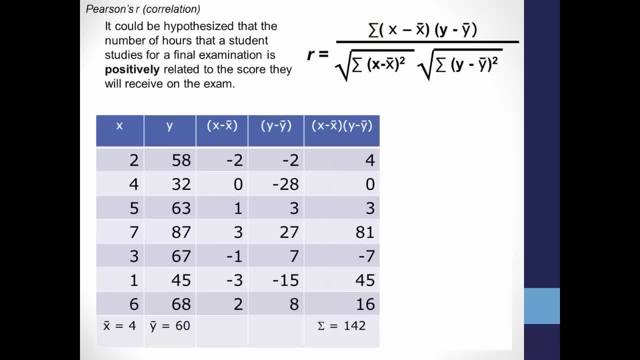 all of these products together, which is 142.. That means that 142 is what goes into the numerator of this formula. Now on to the denominator which tells you to square the result of each score minus the group mean. Go back to this column Negative: 2 squared is 4,, 0 squared is 0, and the rest. 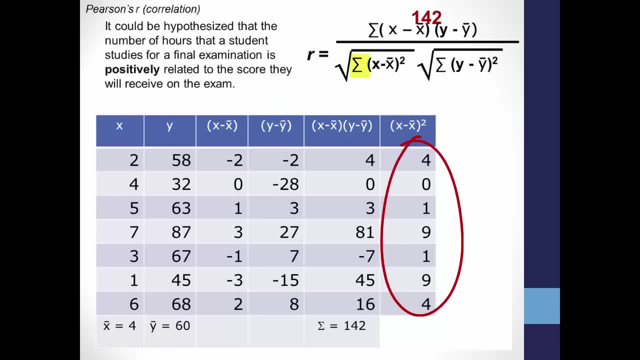 of the x group. Sigma again tells you to add all of these numbers together and we will get 28.. You do the same for the y scores: Negative 2 squared is 4, negative 28 squared is 784, and so on. 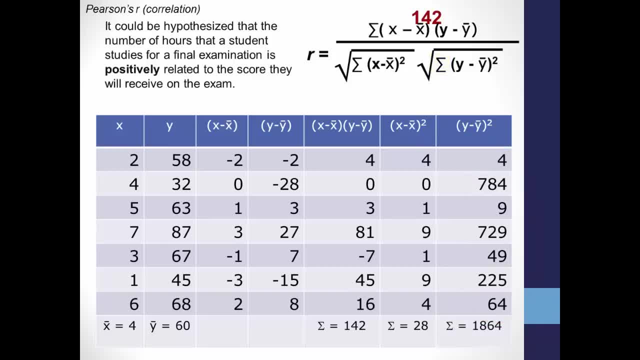 Add them all together and you get 1864.. Now you have all of the data for the denominator. Now it's time to finish off the formula. Just a review of the formula and what we've calculated already. First we have the sigma. 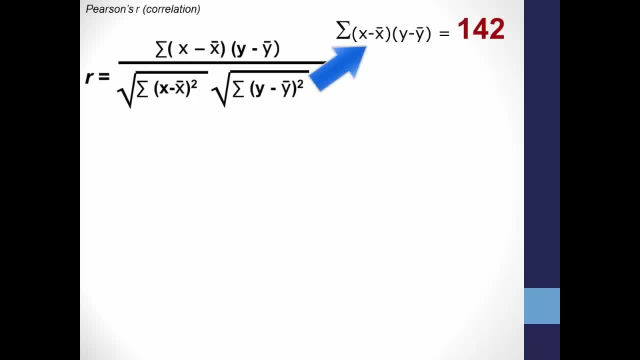 and we have the sum of each score on the x variable minus the mean of the x group, multiplied by the sum of each group on the y variable minus the y variable's group mean, so 142.. You've calculated the sum of each score minus the mean squared for each of the two variables. 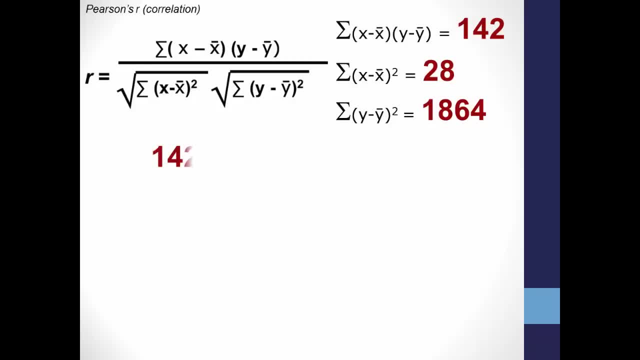 x and y. Plugging that into the equation is 142 divided by the sum of the square roots of 28 and 1864, which is 5.29 times 43.17, or 1.25.. Reducing that down becomes 142 divided by 228.46, and finally, that tells you that r. 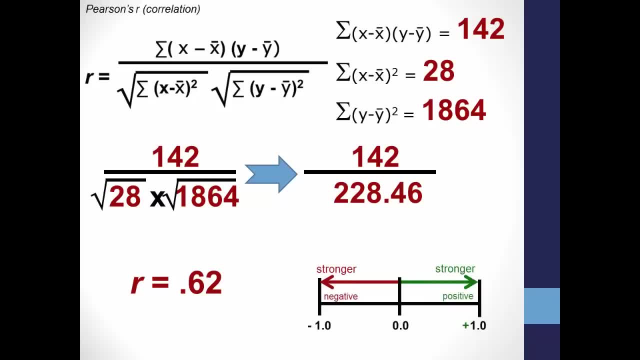 equals 0.62.. What this tells you is that, as 0.62 is close to the positive 1.0,, it appears to be a very strong positive correlation. It appears, then, that the number of hours spent studying for an exam is positively correlated or connected to the exam score. But now we have to take the next step to compute the sum of each score, and that is to calculate the sum of each score minus the mean squared for each of the two variables x and y, squared by the sum of each score minus the mean squared for each of the two variables x and y. 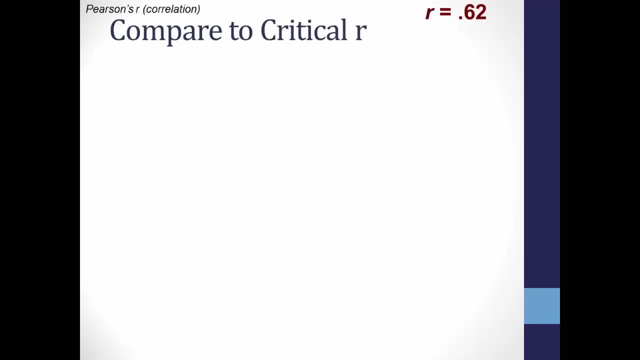 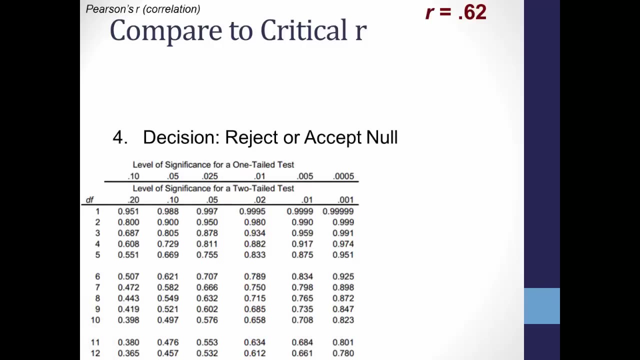 To do this we need to compare our calculated r of 0.62 to determine whether we should accept or reject the null hypothesis, and for that we'll need our critical value table for Pearson's r. First we need to calculate degrees of freedom, which is n minus 2.. Remember that we had 7. 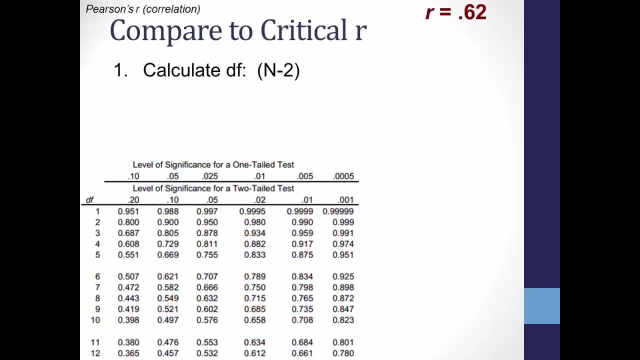 sets of scores: 7 scores on the x variable and 7 on the y variable, for a total of 14 scores. 14 minus 2 equals 12 degrees of freedom, And you'll recall that degrees of freedom refers to how many ways 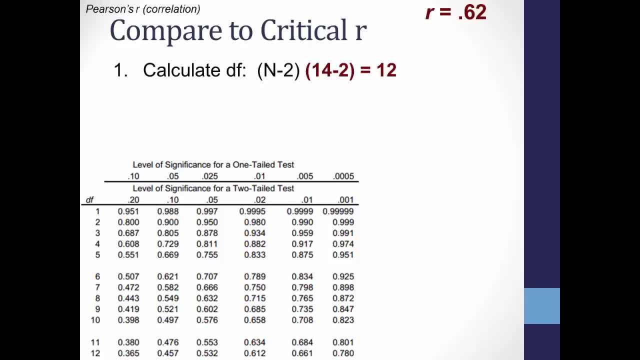 our data could be combined and still produce the same value for a statistic. Assuming an alpha level of 0.05 for a one-tailed test, meaning that we're only willing to accept a 5% chance of error, we can look for critical r. 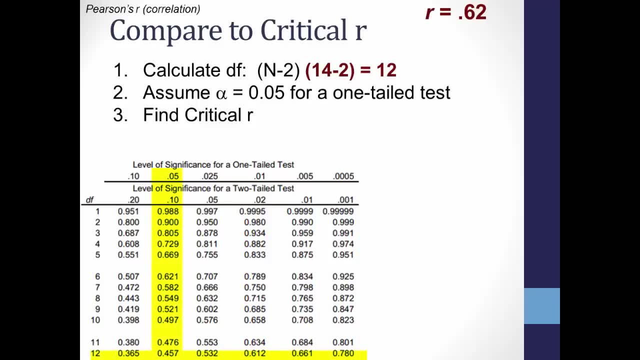 Find where 12 degrees of freedom intersect with a one-tailed test at 0.05, and that's 0.457, our critical r value. Remember that if our calculated statistic is equal to or higher than the critical value, you would reject the null hypothesis, while if it is, 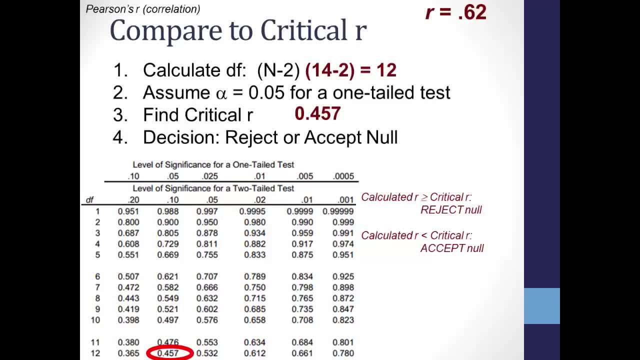 less than the critical value, you would accept the null hypothesis. In this case, 0.62 is greater than the 0.457 critical value, meaning that we reject the null in favor of the alternative hypothesis. We would conclude, then, that we are 95% sure that the number of hours studying 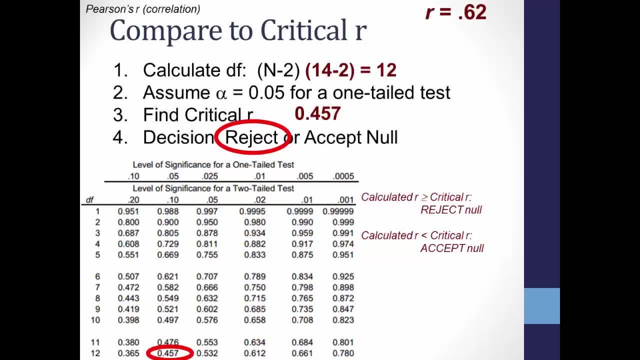 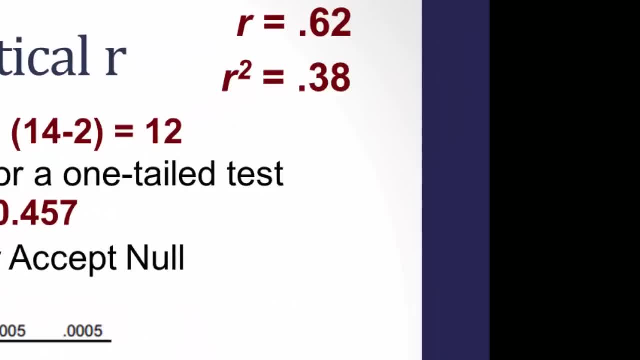 for an exam does in fact positively correlate with scores on the exam. Now we talked earlier about r-squared, which is Pearson's r-squared, and this refers to what percent of the independent variable x, or in this case the number of hours studying, explains what happens to the 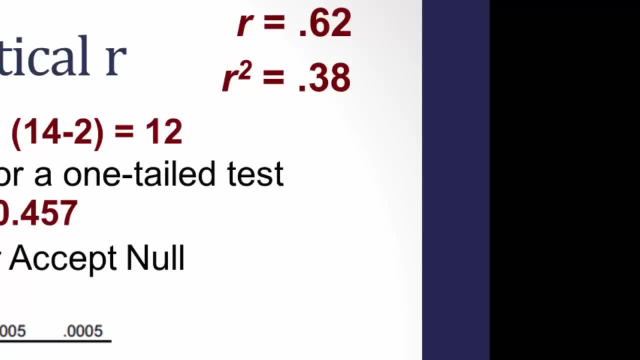 dependent variable y or score on the exam, And in this case it looks like this positive correlation explains about 38% of the variation. Remember that the closer r-squared is to 1, the better x explains y. Processing Time. 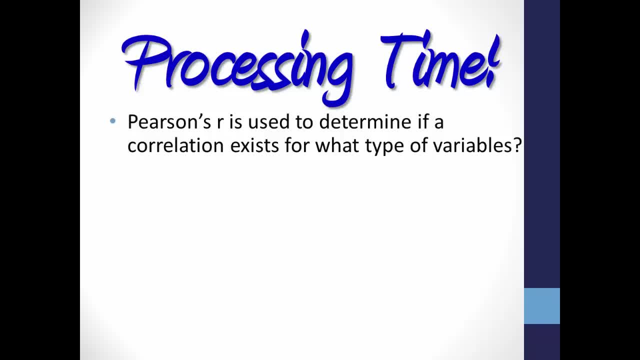 Pearson's r-squared is used to determine if a correlation exists for what type of variables. It is looking for a relationship between two continuous-level variables, such as time spent on a treadmill and calories burned. Which of the following indicates the strongest relationship, as measured by Pearson's r: 0.12, negative 0.68, 0.50, or negative 0.08?? Remember that. 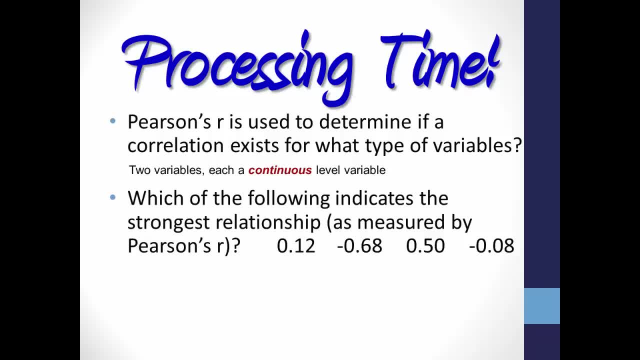 Pearson's r-squared ranges from a negative 1.0,, which is a perfect negative correlation, to a positive 1.0, a perfect positive correlation. The closer the statistic is to 1,, either on the negative side or the positive side, the stronger the correlation. So, of these negative, 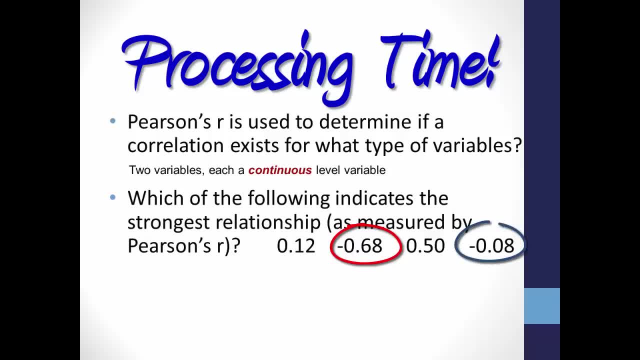 0.68 represents the strongest correlation and negative 0.08 represents the weakest. 如此, What is the difference between Pearson's r and r-squared? Pearson's r-squared is equal to the coefficient of negative 0.08.. In addition, the correlation of r-squared is closer to the correlation of the correlation between r-squared and poor- multimedia variables. Measuring Time, Pearson's r-squared is used to determine when a class is more likely to be connected with negative 0.08 or negative 0.08, or any class that is positive. This is how we can identify the Convention. 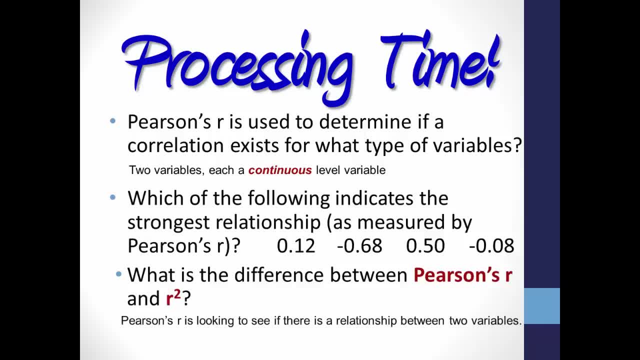 Pearson's R is looking to determine if a relationship exists between two variables and, if so, what type of relationship. R squared used for regression analysis? is the Pearson's R statistic squared used to estimate how much of the independent variable explains what happened to the dependent variable? 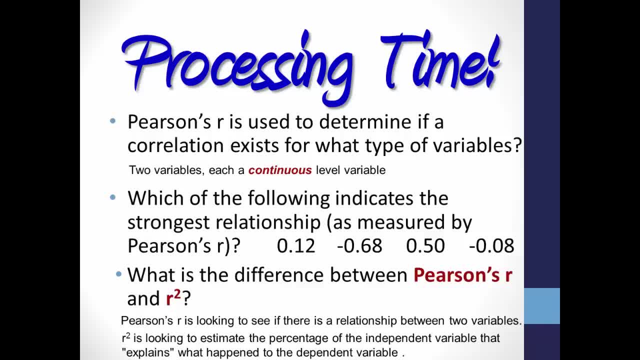 Or put another way, what percentage of the variation in the score on the dependent variable can be explained by the independent variable? And finally, I'll leave you with an off-key song that my statistics professor made us sing in class: Association is not causation. it's often known as correlation. 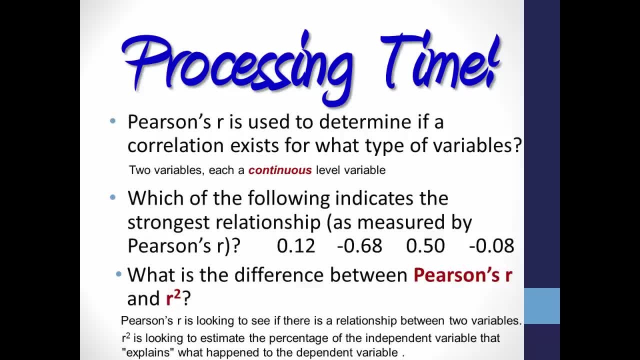 Now you should have a better idea of when to use Pearson's R and with what variables, as well as what the resulting statistic means. You booked a Royal Caribbean cruise and now you're wondering what's included with your cruise fare and what's going to cost extra. Today I'm going to break down exactly what is included with everything you paid for with your Royal Caribbean cruise. Hey everyone, it's Matt from RoyalCaribbeanBlogcom, and one of the most common questions. 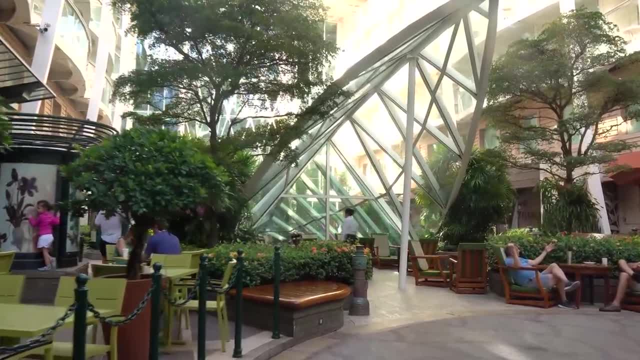 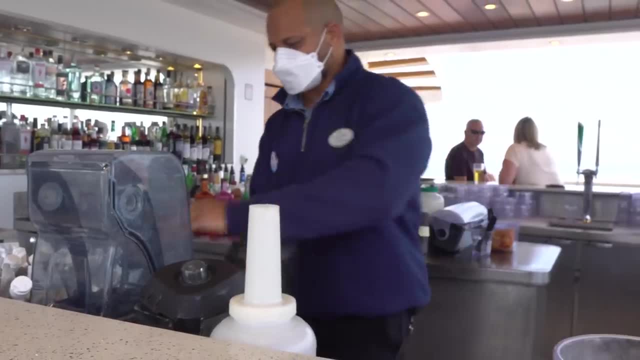 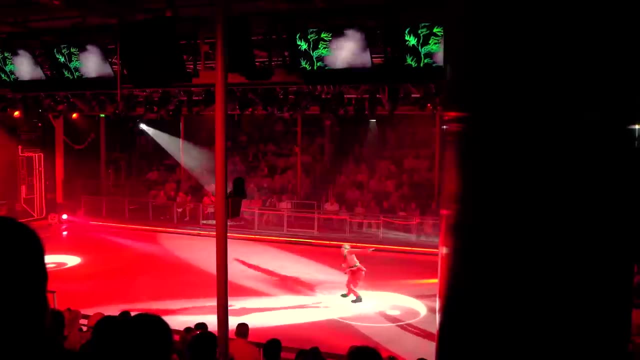 that I ever get about Royal Caribbean is what is included with my cruise fare. There are a lot of components to any cruise vacation and it can be a little overwhelming to understand what's included and what costs extra with a Royal Caribbean cruise. Now the good news is Royal Caribbean includes a lot of activities: food, entertainment. and destinations in your cruise fare. When you consider everything that the base fare includes, it's an excellent value. But Royal Caribbean gives guests the choice of having add-ons to their cruise that they elect to pay extra for, such as drink packages, dining packages. fitness classes, specialty restaurants and more. These add-ons come as an extra fee on top of the cruise fare. So let's break down what's included with your cruise fare and what's going to cost extra, starting off with accommodations, Accommodations, which is your cabin on your cruise ship. 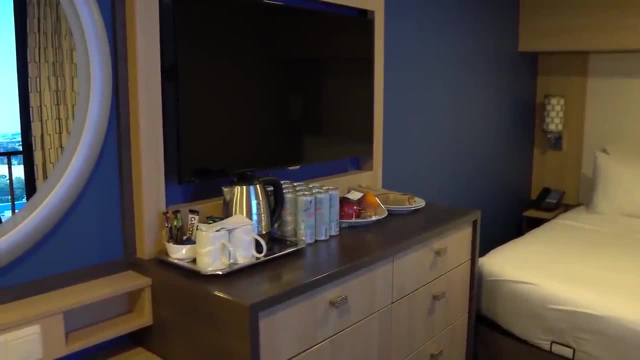 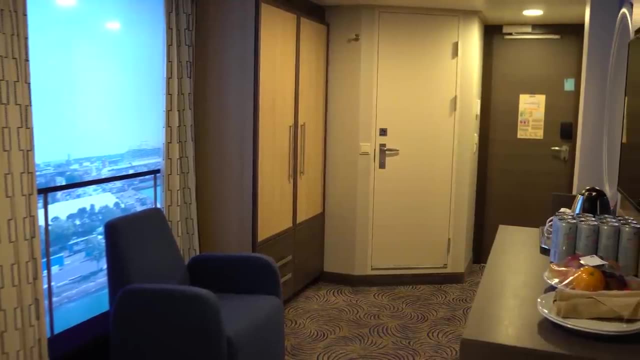 are included with your cruise fare for exclusive use for you. You're not sharing a bathroom with anybody else, or anything like that. Depending on which type of cabin you book, the exact size, amenities and layout of the room are going to vary, But at the very least, 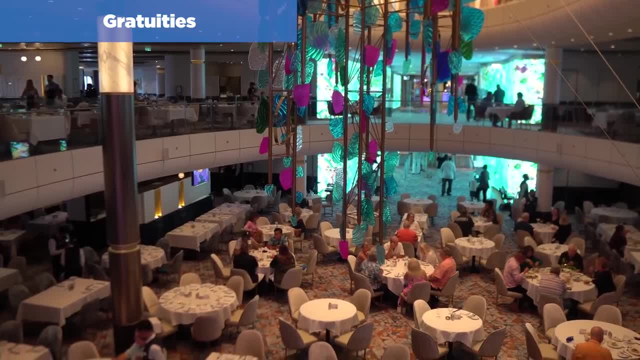 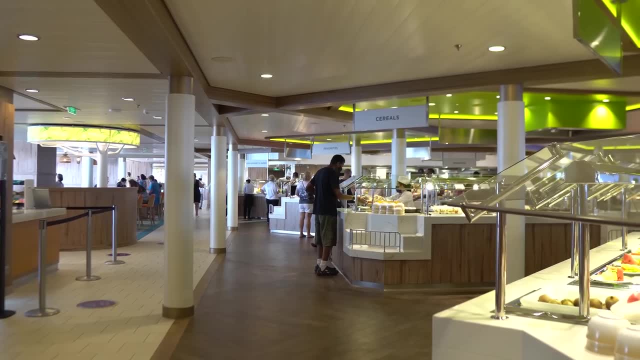 Gratuities on Royal Caribbean have two choices when it comes to gratuities for service-oriented crew on board. You may elect to prepay gratuities prior to your cruise or have gratuities automatically charged on a daily basis to the CPAS account. Cruise fares in some countries like Australia. 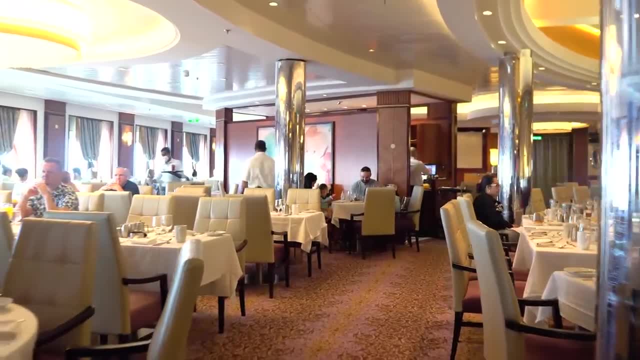 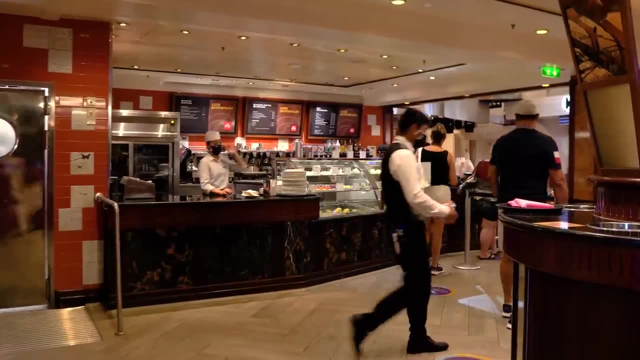 are already included in the cruise fare. As of March 3, 2022,, guests pay $14.50 per guest per day service charge. For guests in a grand suite or above, the amount is $17.50 per guest per day.